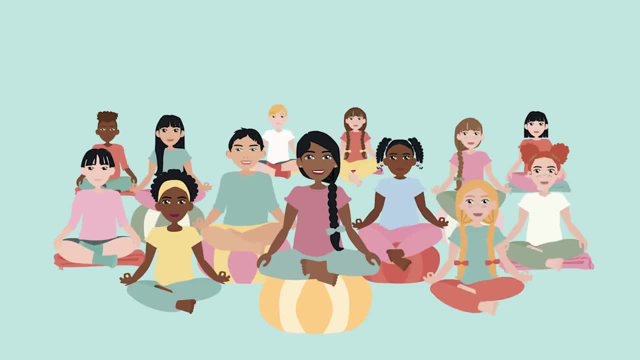 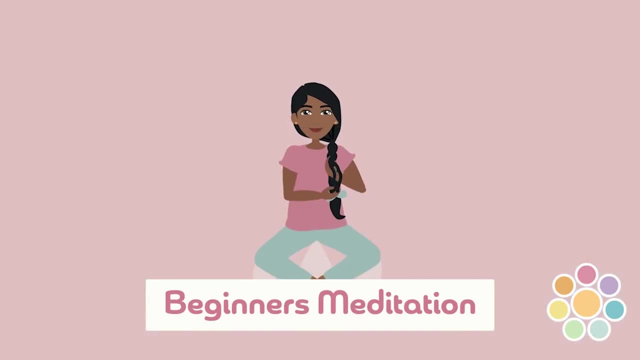 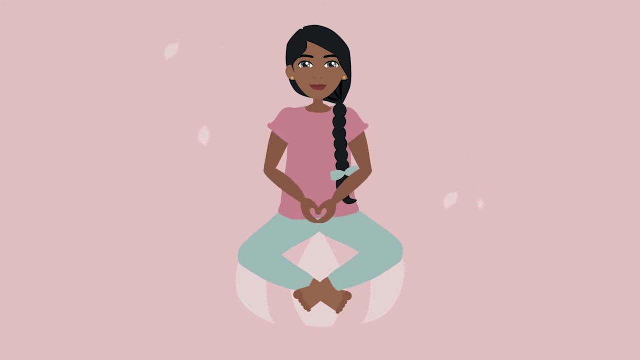 Hello there, Welcome In this quick meditation. we are going to take a moment to check in with ourselves, calm our minds and release some tension. You deserve a little break from your day to focus on yourself. Let's start by getting nice and comfortable. Feel free to sit or. 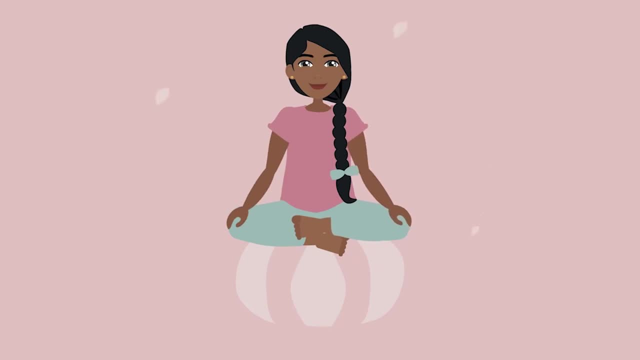 lie down whichever is most comfortable for you. Some even find it comforting to place their hands over their heart. Now that you're comfortable, go ahead and close your eyes. Let's slow down and calm our minds by focusing on our breath. Slowly, take a deep breath in. 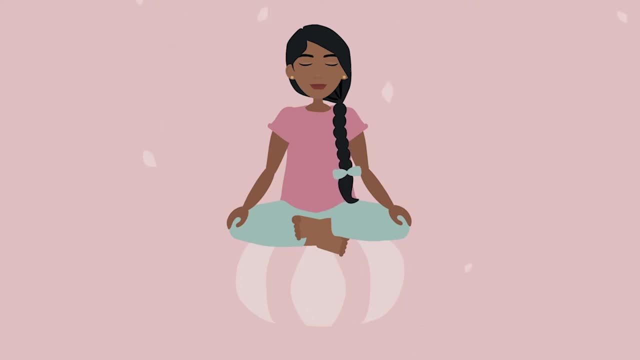 through your nose and breathe out through your mouth. When you breathe in, feel your belly and ribs expand as they slowly fill it there. Deep breath in through your nose and let it out through your mouth. One more time: Deep breath in through your nose and let it out. 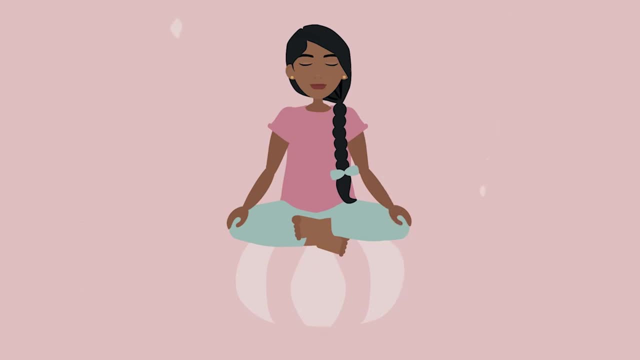 Continue to breathe. Imagine you are inside of a giant, gently floating bubble. Inside this bubble is joy, joy, relaxation and safety. Nothing bad can enter your bubble. You are completely protected. Fill your bubble with things that make you feel happy and calm: Your favorite smells, your favorite memories. 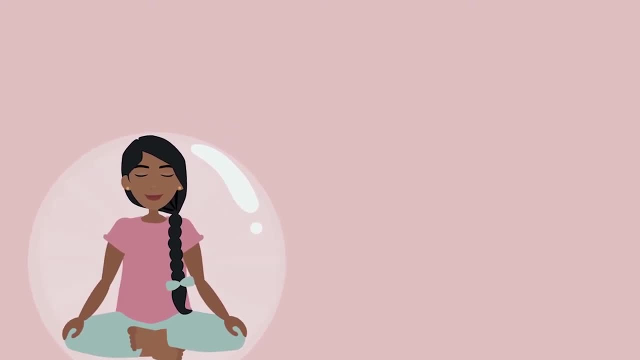 your favorite thoughts. your favorite thoughts, your favorite dreams. your favorite thoughts, your favorite sounds, Your favorite sounds. This is your bubble. It's only for you. Make it your safe place. Take a deep breath in and slowly breathe in all the goodness surrounding you in your bubble. 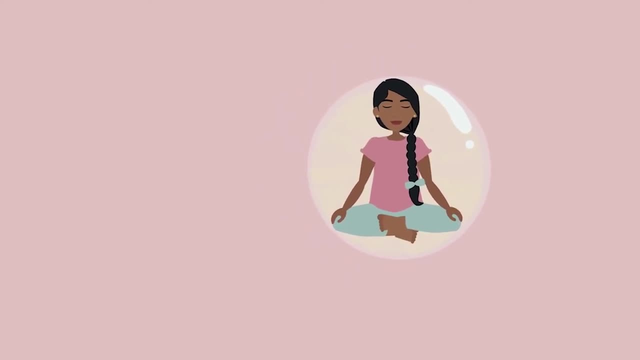 and let it out. Here's another, gracias. Take another nice one right here. Take a deep breath in, out, Continue to breathe. Every time you breathe in, more and more of the goodness surrounding you is filling your lungs and warming your heart, And every time you breathe out any. 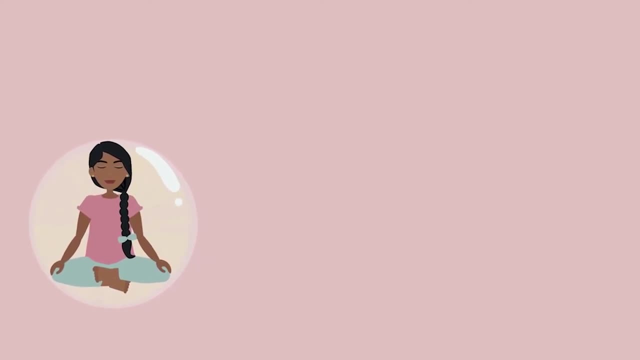 stress or worries, immediately exit your bubble. There's only room for good in your bubble. Sometimes we unknowingly hold on to tension in our bodies, and that's okay. Let's release some of that tension. Relax your forehead And unfurl your eyebrows. 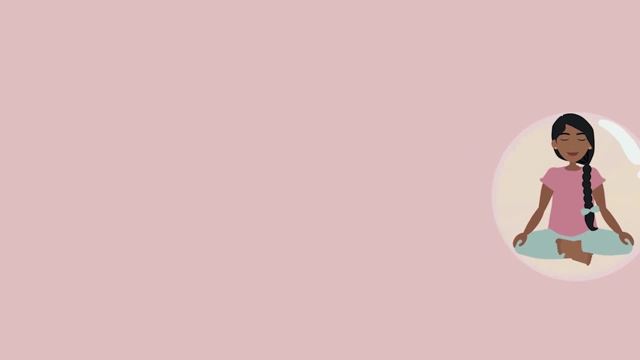 Release and relax your jaw, Lower and relax your shoulders and back, Relax your arms, hands and fingers. Relax And relax your chest and stomach, And relax your legs, feet and toes. Now your whole body feels lighter. Every time you breathe in, feel your body becoming more and more warm.